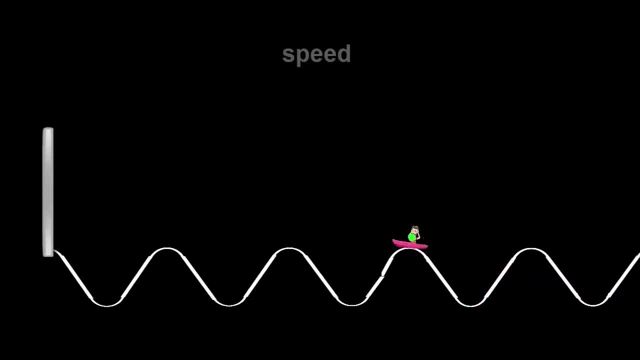 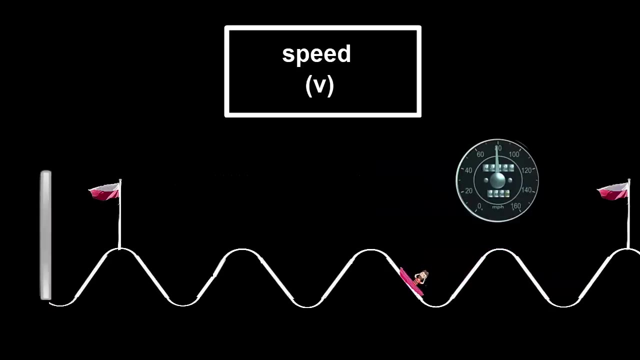 You can check this out next time you're in a boat. The speed of a wave is how fast it's travelling from left to right here and is usually given the symbol V, which stands for velocity. Velocity is another word for speed. Notice how the speed of the wave is constant. 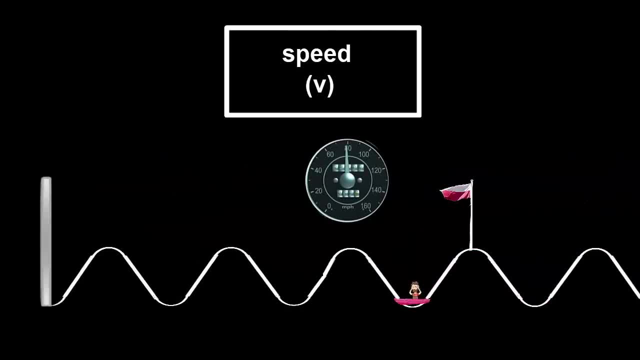 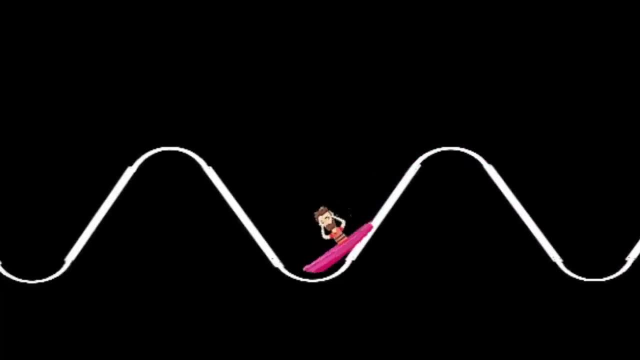 And each crest moves at the same speed as the others, But the boat's up and down speed changes and you can see that it's moving fastest in the middle of its cycle. This cyclic type of movement is called simple harmonic motion and we'll cover that later. 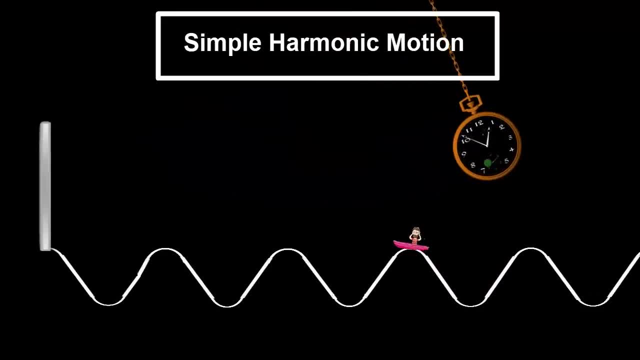 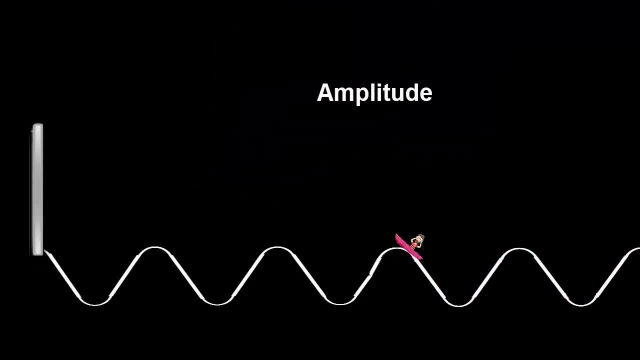 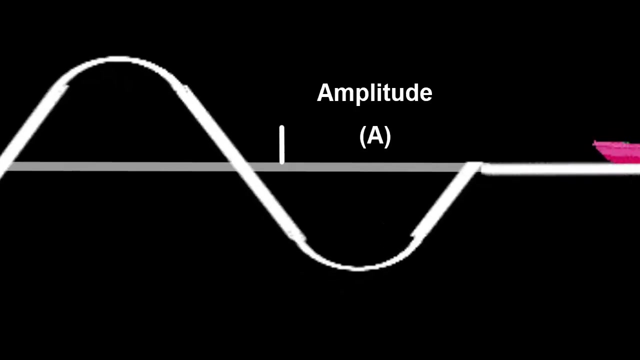 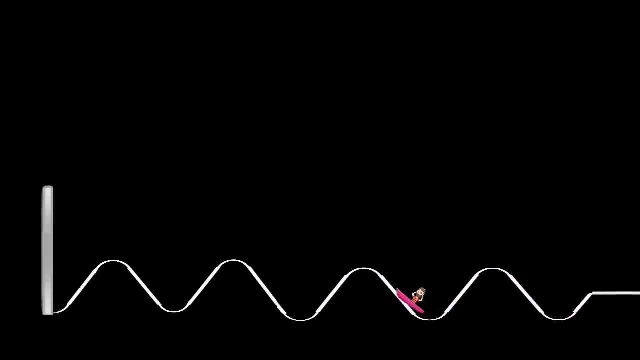 A pendulum is another example of simple harmonic motion, so it moves horizontally instead of vertically. The amplitude of a wave with symbol A is how high it moves up and down. compared to a flat, calm surface, Higher amplitudes are caused by the source having more energy. 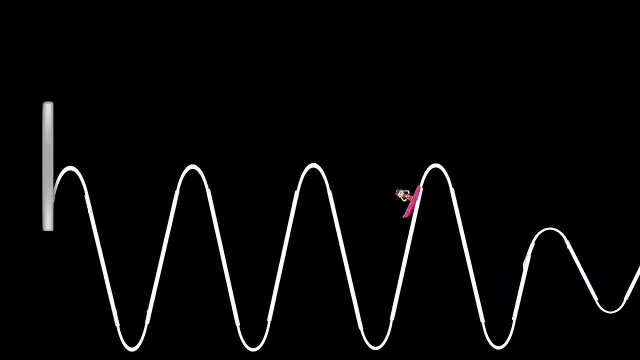 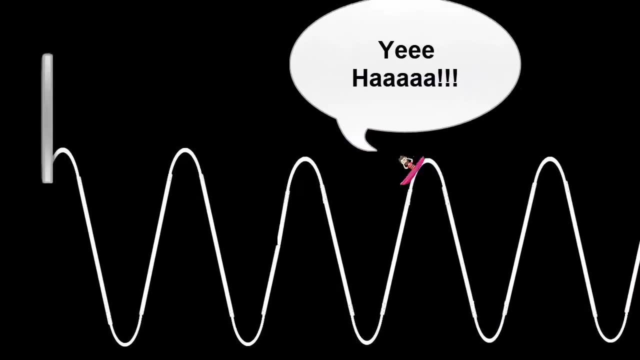 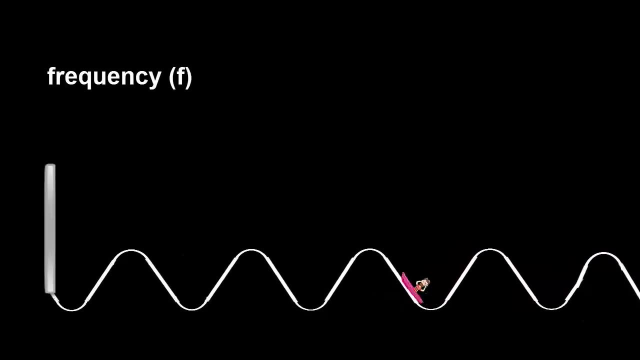 and dipping further into and out of the water. The guy on the boat would notice that he would rise and fall more, so he'd get a more energetic ride. The wave's frequency, given the symbol F, is the number of waves being made each second. 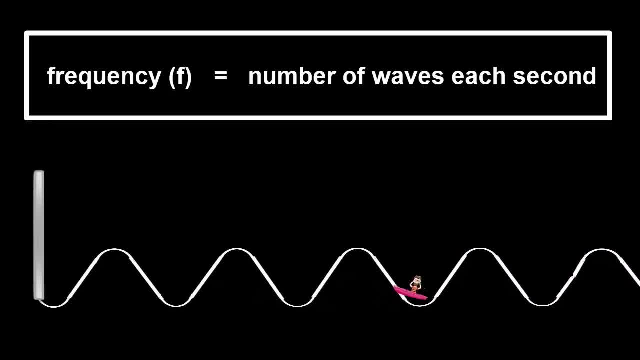 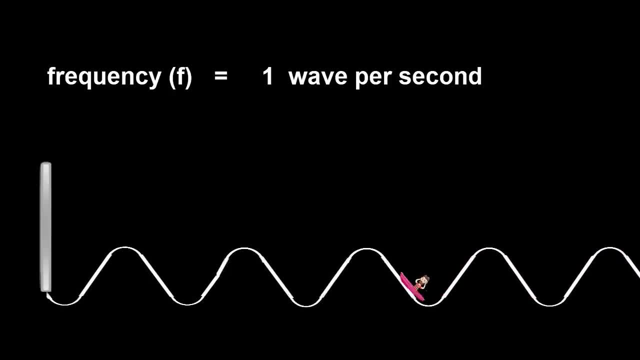 The frequency is also the number of waves passing by the guy in the boat each second. Here only one wave is passing per second, so scientists say that its frequency is one hertz. Hertz is the unit of frequency and it just means waves per second. 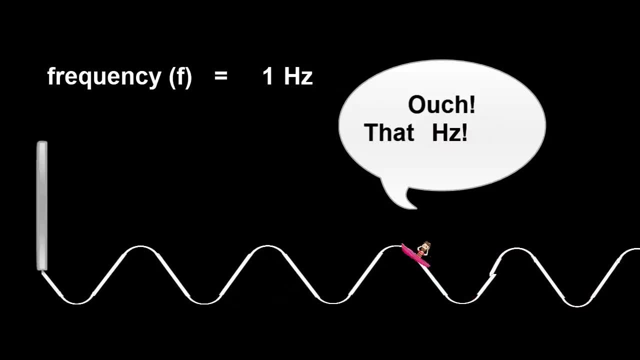 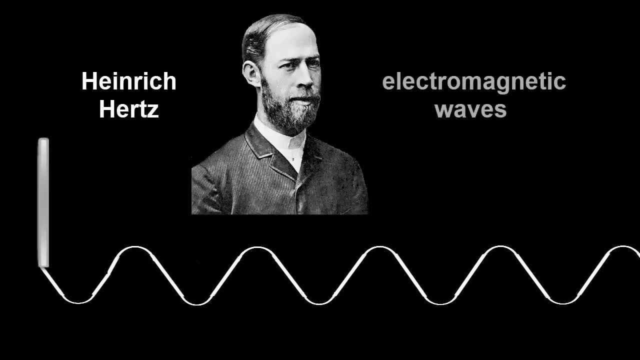 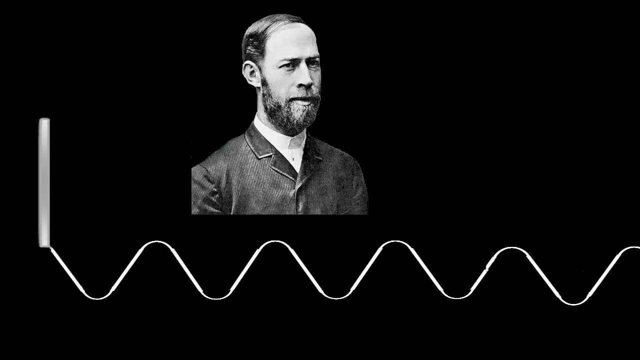 It's usually shortened to HZ. This unit was named after the famous German scientist, Heinrich Hertz, who proved the existence of electromagnetic waves, which we'll explain in another video. Interestingly, Hertz was not only a clever scientist, he could also speak Arabic.